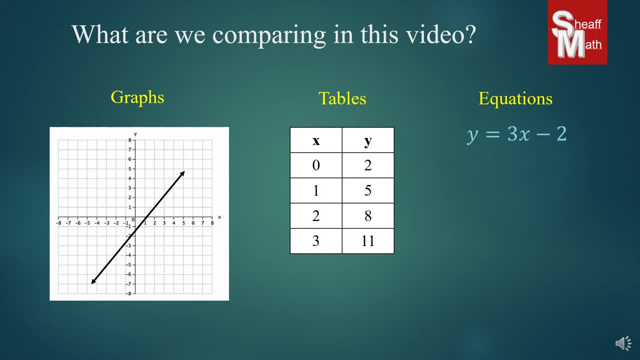 to compare these different three. So the best way to learn how to compare them is to be able to find the important information about these three. So there's three pieces of information that are crucial for comparing linear functions. The first one is the slope. 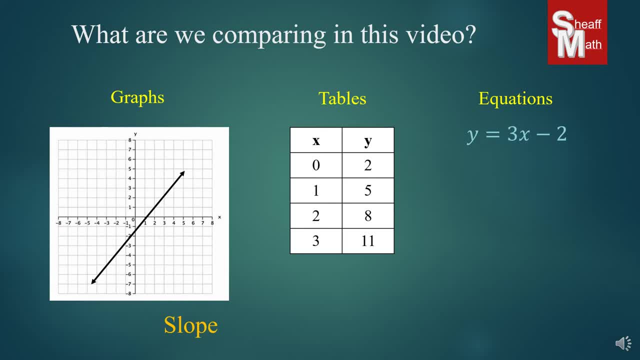 The rise over the run, The rate of change, The y intercept where that line goes through the y axis, or the zero term, And also f of x. This is what you're going to also be asked to find sometimes. And f of x is simply: if x equals three, what does y equal? The function of x? 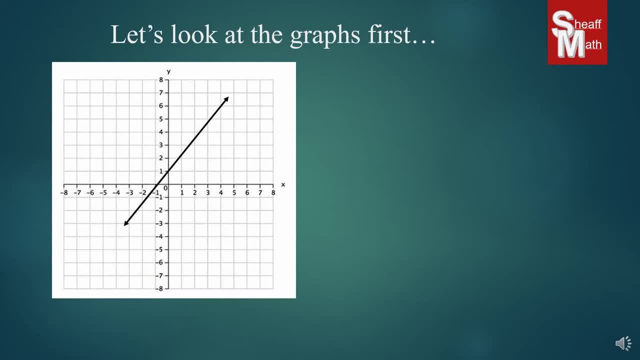 All right, let's look at graphs first, And when we're trying to find those three key pieces of information, the easiest one to start with, I think, is the y intercept, Wherever that line is going through the y axis. that's the y intercept And R's- if you look, it happens to: 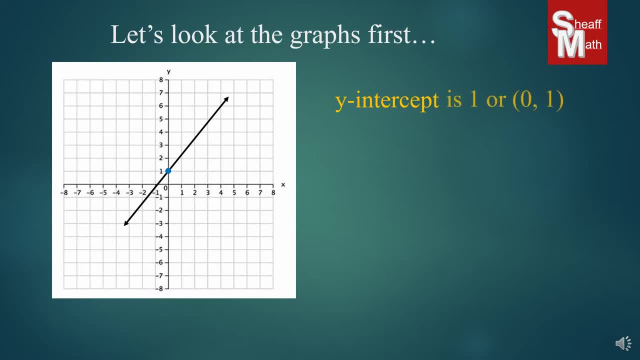 be going through one, And so our y intercept is one. Or in the point form you would put zero one. Now the slope: In order to find the slope, you have to find two really good points on your line. You have to make sure both of the points are. 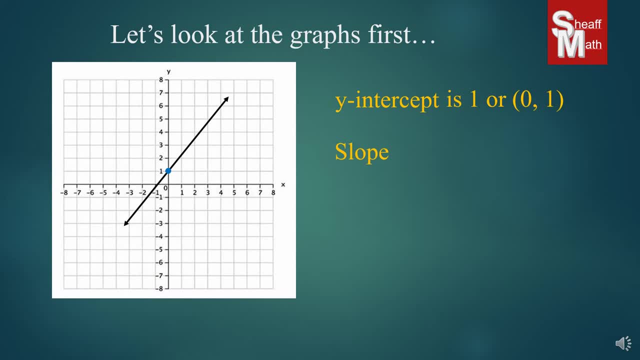 going through really nice crosshairs, or lattice points as we call them, And so, looking at this one, I can see that the line is for sure going through four six as well. So with these two points- zero one and four six- I'm going to find the rise and the run. Is it going up or down? And 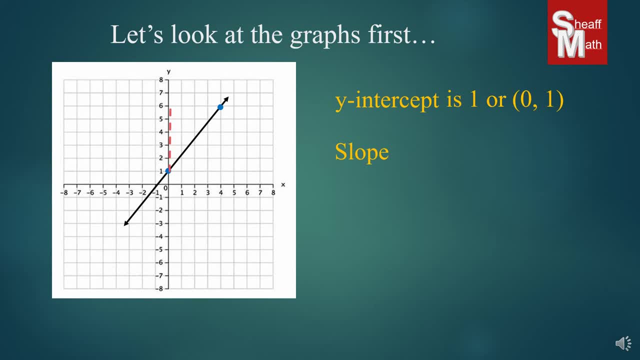 then over to the right. So this one is going up by five and over four, And so it doesn't matter which points you pick, it's always going to go up five over four, And so five over four is our slope. Sometimes your slopes come out to whole numbers, sometimes fractions. 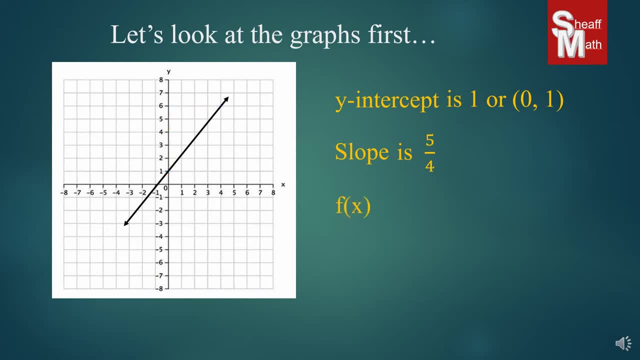 That's okay. Now, the last thing you might be able to find out is f of x, And so that would be something like this: What is f of four? In other words, if x equals four, what does y equal? So let's find four. 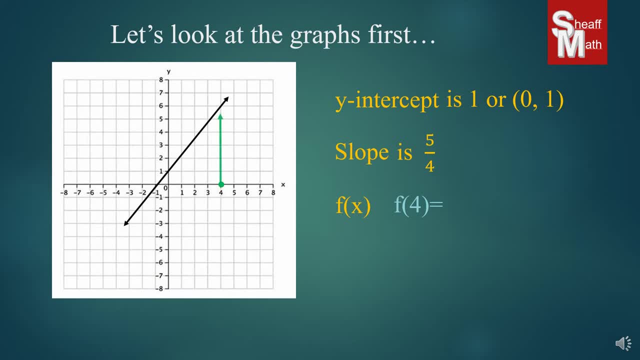 in the x-axis. There it is right there in green, And let's go up to see where the four in the line meet, And it meets right there, And so the y would be six. So f of four equals six, And so finding these three pieces of information in a graph is pretty easy. 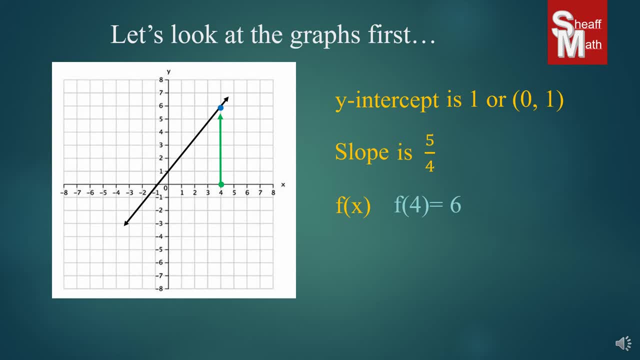 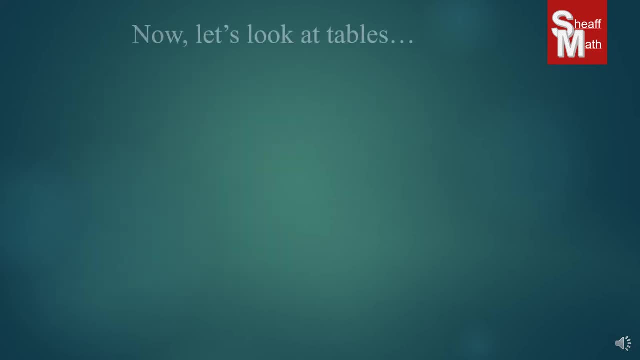 You just have to look at it, find the rise and the run, and then just kind of find the points that are necessary. Now let's look at a table. Now this particular table is a very easy table. There are a few reasons why, And I put an easy one in here just to give you an idea of what we're looking for. 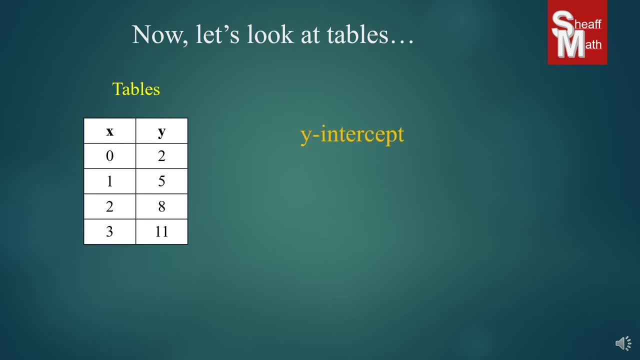 So the first thing we're finding is the y-intercept And the y-intercept. that initial value is the zero term. So when x is 0, that is the y-intercept, So ry happens to be 2.. And so you could say: the y-intercept is 2 or the point is 0,. 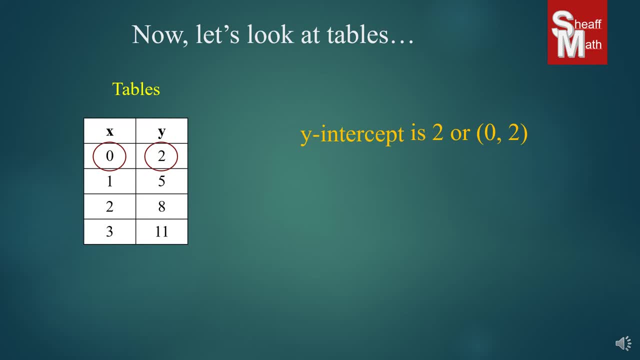 too. It's really easy to find out if you have that zero term there. Now let's find the slope. Now, the first thing we have to look at is: what are the x's are going by on the left, And you can see they're going up by 1.. This is the perfect. 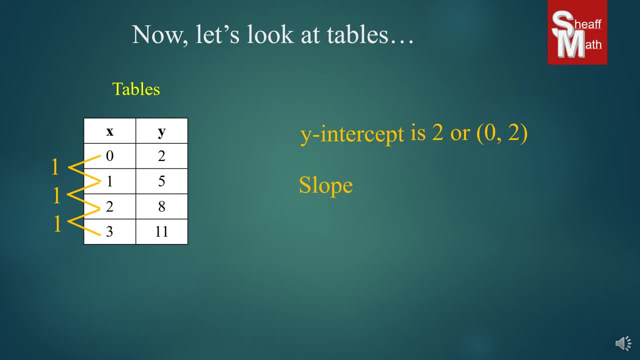 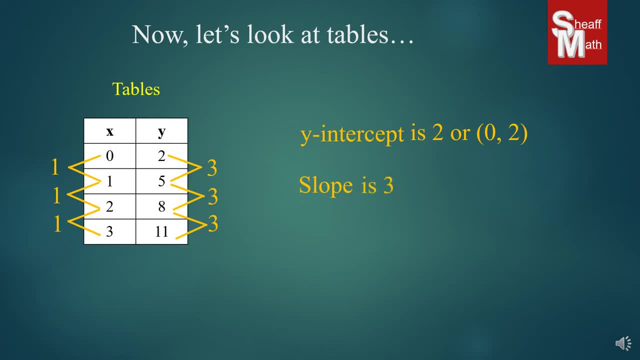 over one equals three. Now, sometimes you'll be asked to find f of x, So let's see f of four right here. Well, we don't have four on our table, but it's close enough to where we can kind of just. 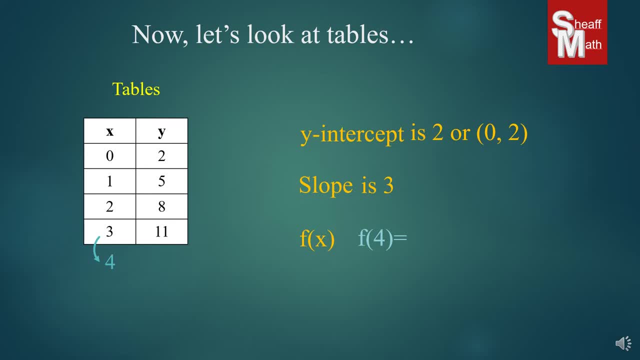 put a four right below there And we know it's going up by three. So 11 plus three is 14.. So when f- I'm sorry, when x- is four, the y equals 14.. So this is a very easy table We're going to. 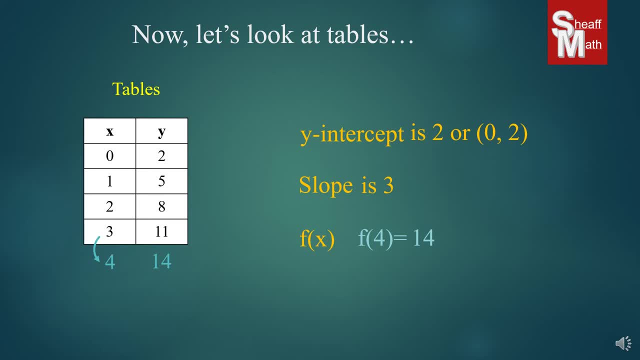 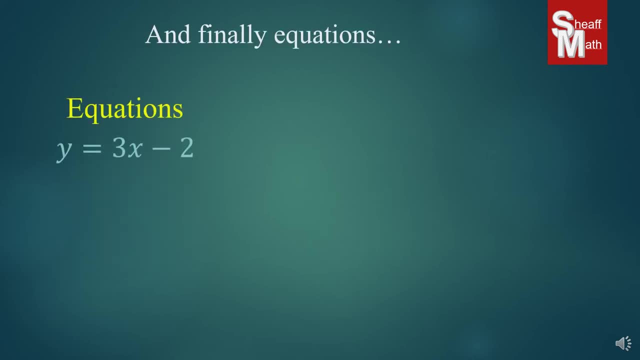 talk about how tables can get a little bit confusing a little bit later. So let's go on to the next one: Equations. So you have a table, You have this equation in slope-intercept form, And these are actually the easiest to find. the 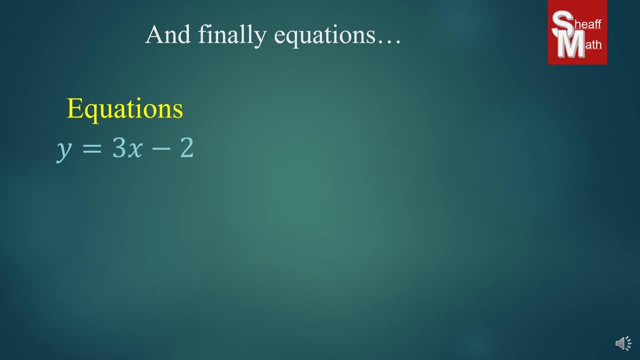 three key pieces of information. Who would have thought that the equation would be the easiest way? Now, we'll find the slope first And, if you remember, this is in slope-intercept form, And so the m is the slope. So whatever number is in that position, the coefficient of x, that is our slope. 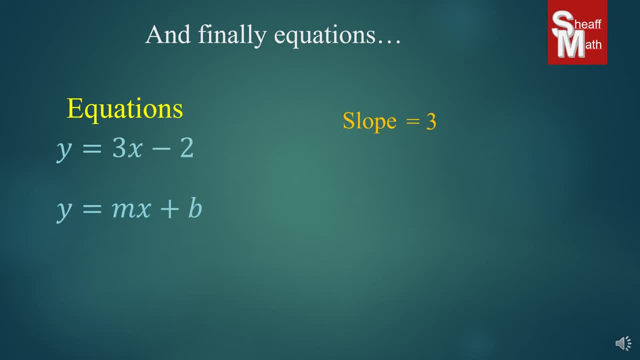 So our slope happens to be x, And so we have this equation in slope-intercept form, And so the m is the slope. So whatever number is in that position, that is our slope. The coefficient of x is two. Now we're going to find the y-intercept, And, as you know, the b is the y-intercept. So whichever, 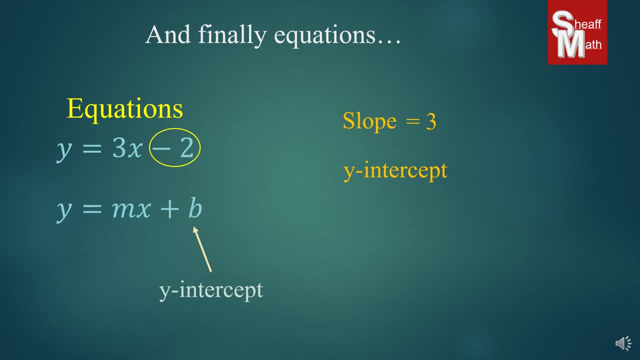 number is in the b position. in this case it's negative two. That is our y-intercept. It's negative two. Now what if we were asked to find the function or the f of x? So let's say we were. 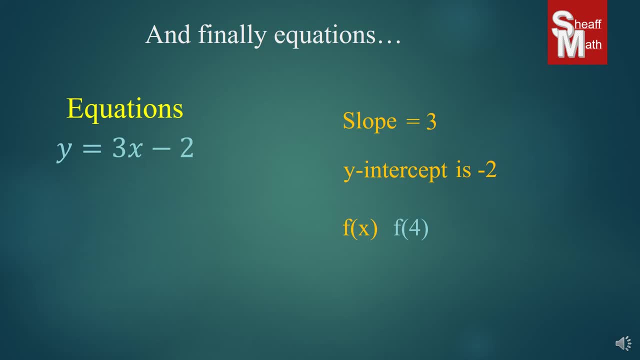 asked to do f of four. So we simply, if f of x is negative four, we're going to find the y-intercept: x equals 4, we're going to put 4 in for x, We're going to substitute it in there and 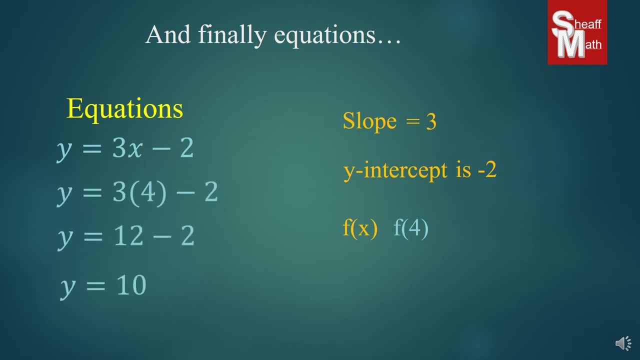 just simplify: 12 minus 2 is 10, and we found our y. If x equals 4,, y equals 10.. So again, the equations, when they're in slope-intercept form, are pretty easy to find, those three. 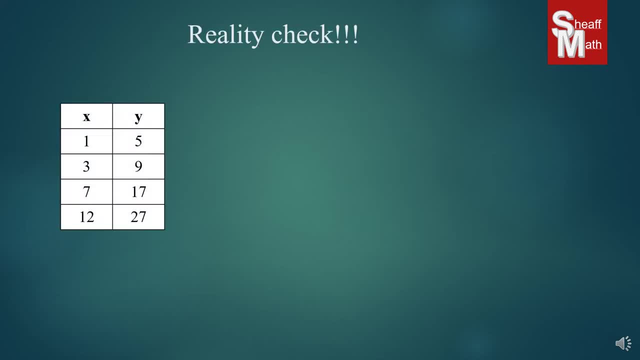 pieces of information. Now I'm going to give you a reality check On the problems that are often given on computer programs. the tables are not that nice If you look at the x's here. if we wanted to find the slope here, look at what's happening to the x's- It goes. 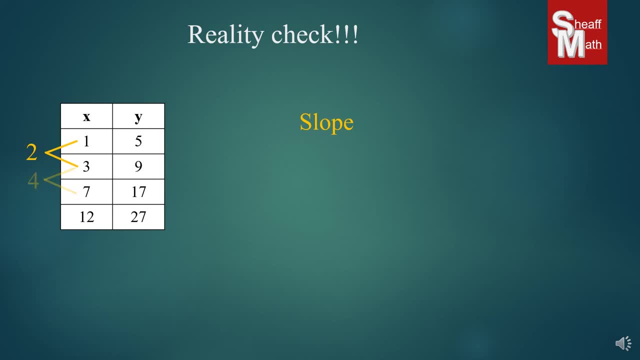 from 1 to 3,, that's up by 2, or over 2.. Then it goes up 4, then it goes up by 5.. That's a real problem. Remember the table we had before. they went up by 1's. So let's look. 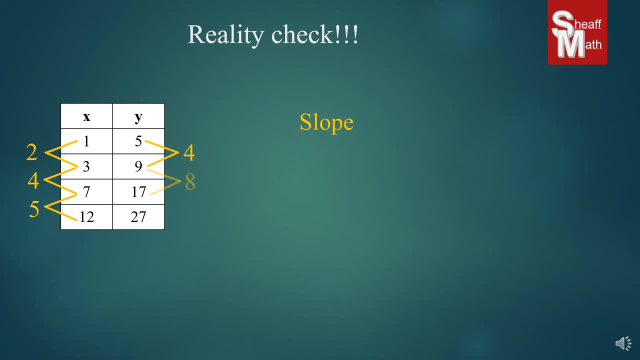 at what's happening on the y side. It's going up by 4,, going up by 8, and going up by 10.. Now, how in the world are you going to find the slope here? Well, I'm going to let you in on a little secret. I want you. 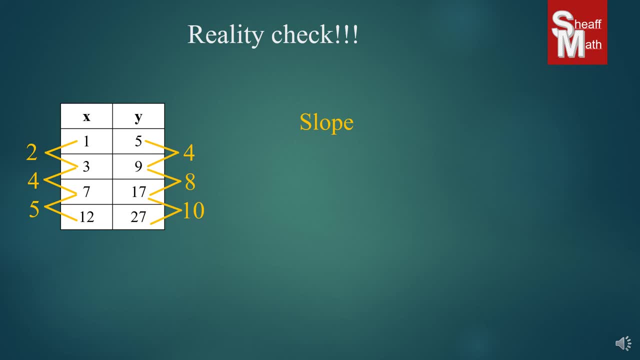 to look at the 4 and the 2. on the first two pairs, 4 is the rise and 2 is the run. So rise over run 4 over 2, is our slope. Let's look at the next one: 8 and 4.. 8 over. 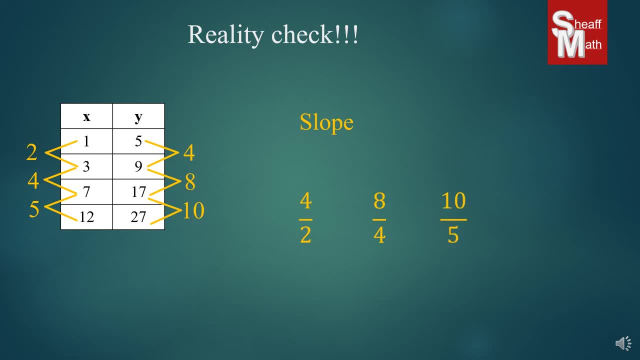 4 is our slope And 10 over 5 is our slope as well. Now, these are different, aren't they? But they're really not. They're the same: 4 divided by 2,, 8 divided by 4, and. 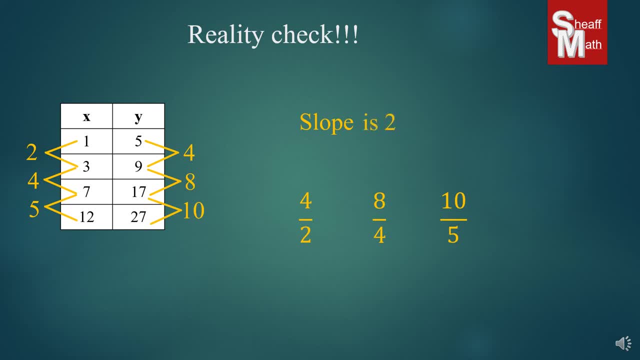 10 divided by 5 are all 2.. So this is a real easy way and you really don't need to do all three of them. You just have to do the first two. If it truly is a function, it's going to have the same slope, no matter how many times you do that. So that's a little. secret. I'm letting you in on that. So let's look at the next one: 8 and 4.. 8 over 4 is our slope, And 10 over 5 is our slope. Now, these are different, aren't they? But they're. really not. These are the same function. And 10 over 5 is our slope, And 10 divided by 4, 8 divided by 4, 8 over 5 is the same And 10 over 5 is the same. So let's look at. these. This is a little secret. They're the same. And 10 over 5 is the same. So let's look at the next one: 8 over 5 is the same. So let's look at the next one: 8 over 5 is. 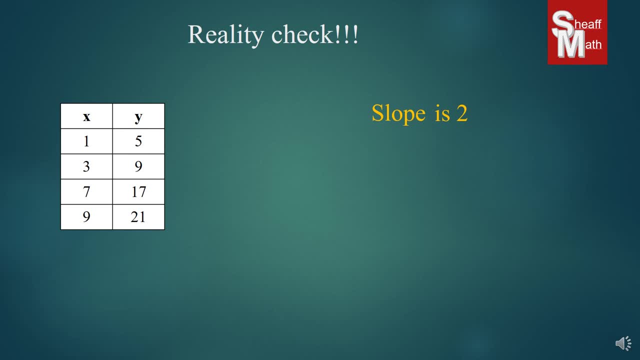 the same. So let's look at the next one: 8 over 5 is the same, So now let's take a look at the y-intercept. We know that our slope is 2, but we don't have a zero term, So I'm 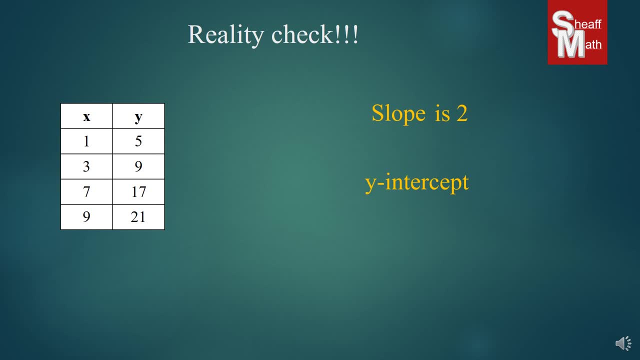 going to have you guys try something. I want you to make a new x-y table, But this time I want you to have all the x's go from 0, 1, 2, 3,, 4,, 5,, 6, 7.. Now, why did I do that? Well, 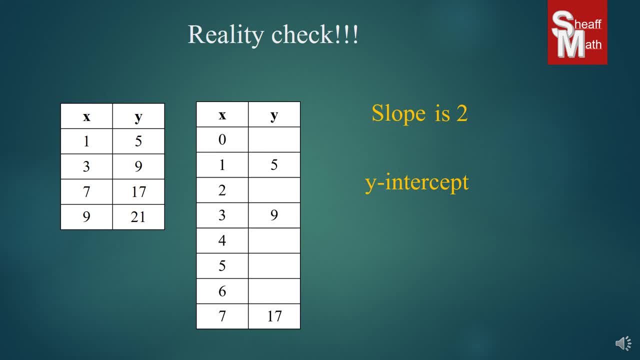 because when they're going up by 1, it makes it a lot easier to understand. And so, if you see, I filled in the 1, 5 and the 3, 9 and the 7, 17.. I didn't even bother to put in the 9, 21. 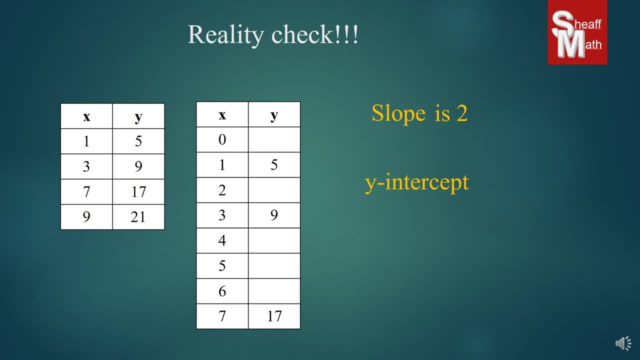 because you really don't need it. All you really need is two points to make this. And so, because we know our slope is 2, if I start at 5, it's going to be going up by 2 each time, So it goes.